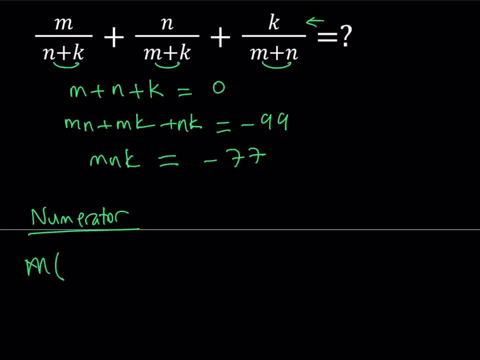 multiplied by. I will have m multiplied by m plus k, m plus n, And then I'll have n multiplied by n plus k, m plus n, And then, finally, k will be multiplied by n plus k, m plus k. Let's go ahead. 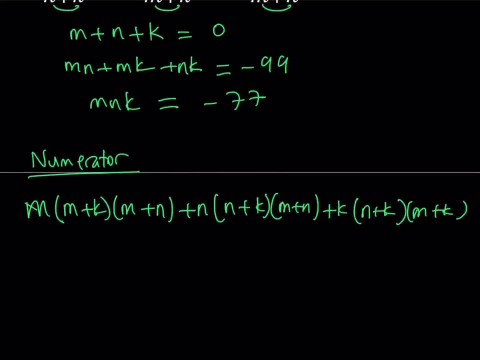 and simplify this first, so you don't have to write the fraction every time. So when you distribute this expression, to keep a long story short, you're going to get something like this: m multiplied by m squared plus mn plus km plus kn. And then we're going to get similar terms from here, like n will. 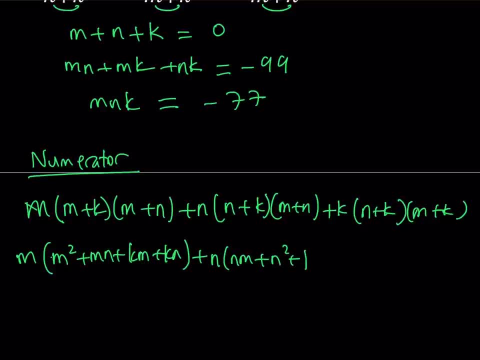 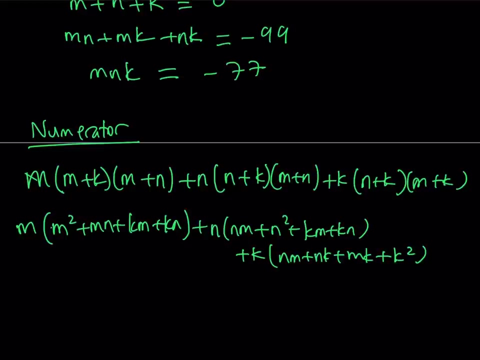 be multiplied by nm, n squared, km and kn, And then we're going to have the k being multiplied by nm, nk, mk and finally, k squared. Now notice that we are getting the same terms here, So some of these terms are going to repeat. 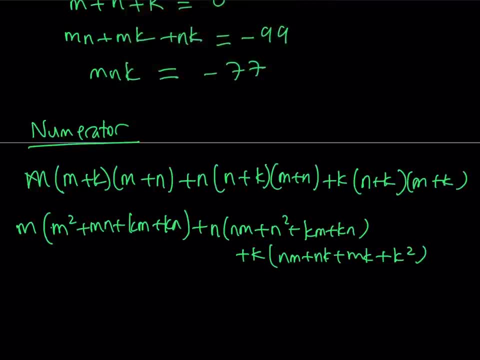 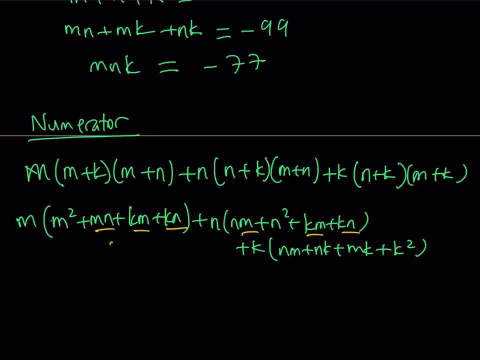 So, for example, if you look at this carefully, I was going to use that color- we have mn, km and kn like these. They're just going to repeat right, So we can basically take out that expression here, and then we're going to have n multiplied by nm, n squared km and kn. 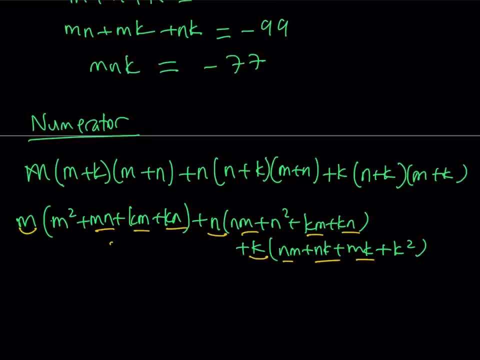 And then we're going to take that as a common factor and multiply, since they're being multiplied by mn k. so we have the following: m plus n plus k is being multiplied by mn plus mk plus nk. Okay, so that's the first part, And then what is left? we multiply m times m squared, which is m. 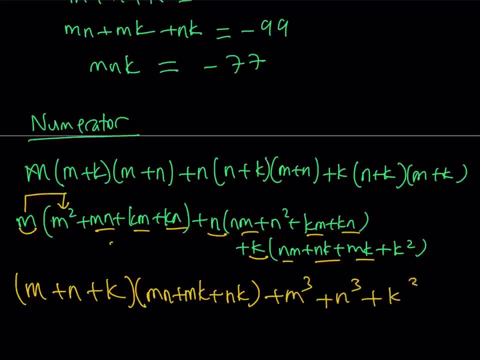 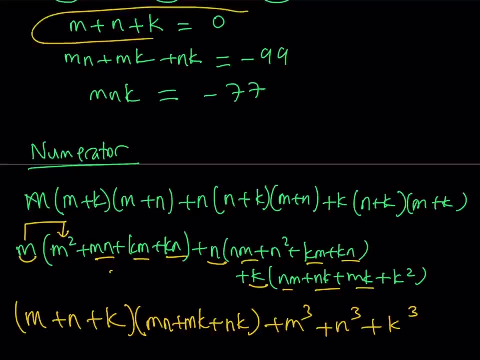 cubed, and then we have n cubed and then k cubed. Now this is the numerator. We haven't done the denominator yet, But notice that this relationship gives us that, okay, m plus n plus k is equal to zero. So I could go ahead and use that. 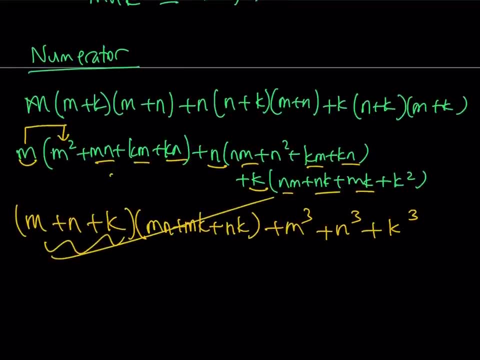 Let's substitute. This whole thing is going to be zero. So by numerator. my numerator is going to be this expression right here: m cubed plus n cubed plus k cubed. Let's save it for now And let's go. 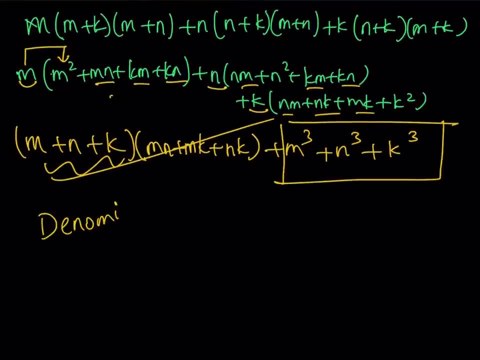 ahead and simplify the denominator, And then we'll put it together and write our fraction. And did I tell you that I'm going to introduce two methods? This is the first one. Okay, So in the denominator we basically have m plus n. 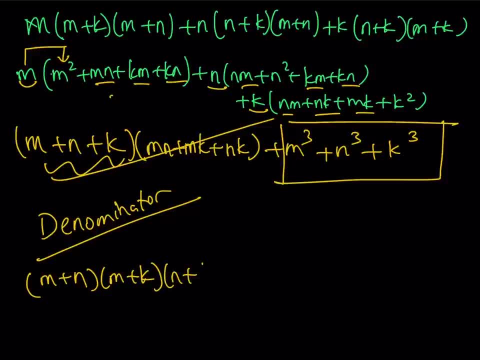 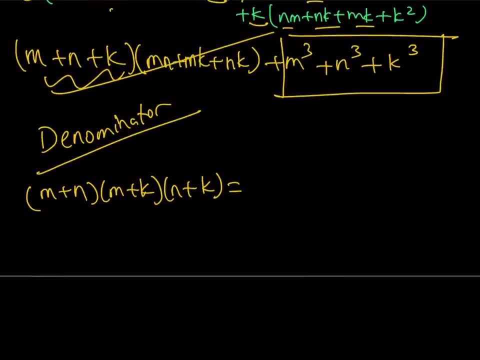 multiplied by m plus k, And that is multiplied by n plus k. Okay, great. Now when we distribute this, obviously we're going to get something like this- Let me go ahead and write that down here, because I don't think it's going to fit: We're going to get something like m squared n. 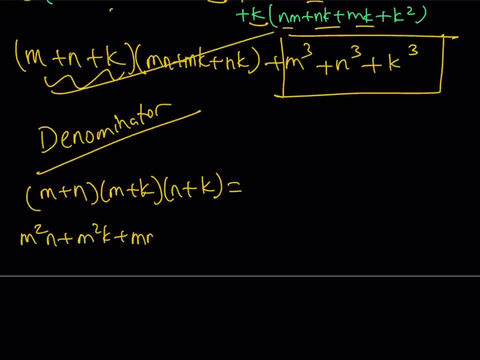 plus m squared, k plus mnk plus mk squared plus mn squared plus mnk, And now we'll have kn squared and nk squared. Okay, so we're supposed to have eight terms here, because two times two times two is equal eight. So what you can do is you can distribute these two first and then distribute them m plus n. 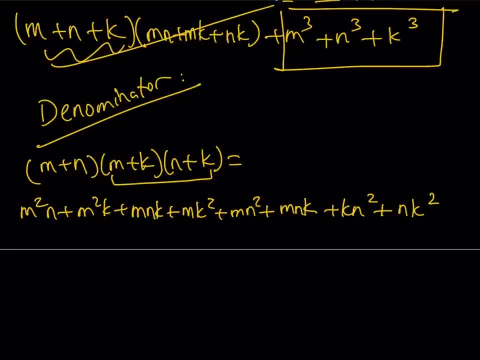 Now we're going to factor the denominator in a special way. So this is what I'd like to do: Bring some of these terms together. For example, I'd like to pick m squared n, mn squared with an mnk. So if I take out mn as a common factor here, I'll be getting m plus n plus k, right? 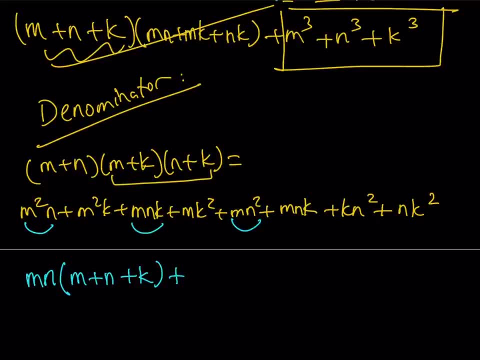 That's cool. Now I'll do something similar for m squared k and mk squared and mnk. So that's going to look like mk times the quantity m plus k plus n. So pretty much they are the same thing. But notice that we don't have an mnk here. But no worries, we're going to take care of that. So I'll be. 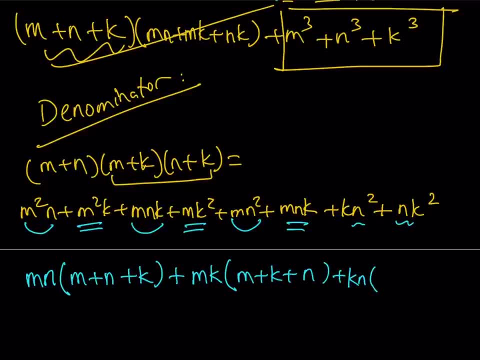 taking out kn, or you can write it as nk- doesn't really matter- And this is going to give you n plus k, But I'd like to have an m, so that we follow the same pattern. But notice that I'm introducing an extra term, which is mnk, So I have to subtract it. So then, 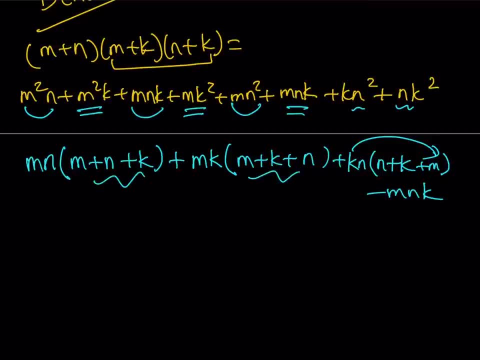 the picture will be complete. Now notice that this is a common factor: m plus n plus k. So let's go ahead and take it out And now from here we're going to be getting mn plus mk, plus nk or kn- doesn't really matter, Of course- minus mnk. So we kind of got an identity, if you ever. 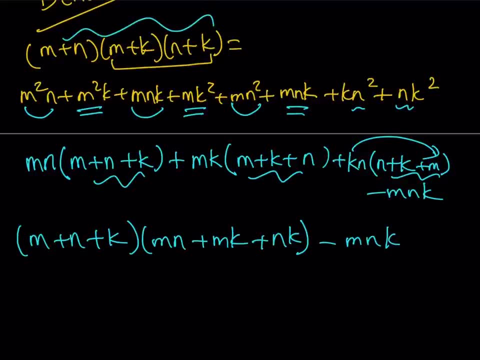 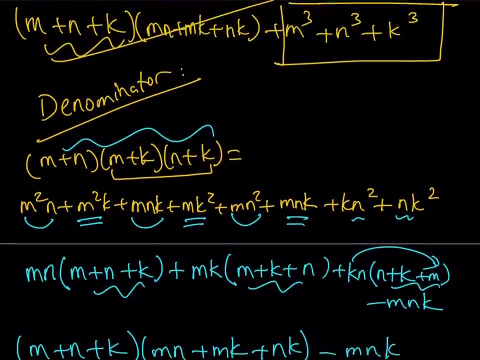 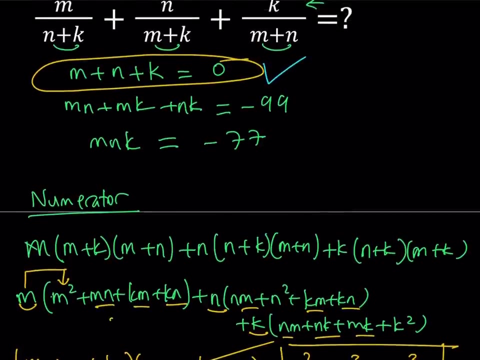 get something like this, because these problems kind of come up on math competitions, sometimes competitions like AMC, And this will be helpful. Anyways, we know that m plus n plus k is zero. You see how useful that information is, Because we know that we don't have b here, So we don't. 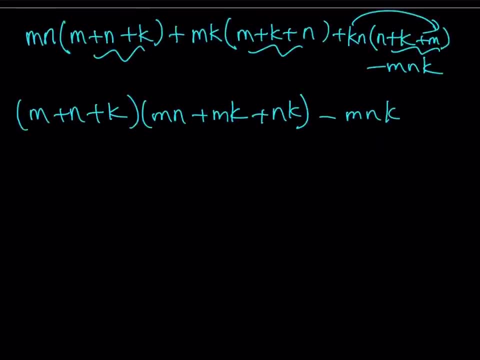 have the x squared term. That's why that's zero. So, since this is zero, what that's supposed to mean? Well, the whole thing is going to be zero. So our denominator is going to be negative. mnk So great. So now I got the numerator. Remember, the numerator was this one. 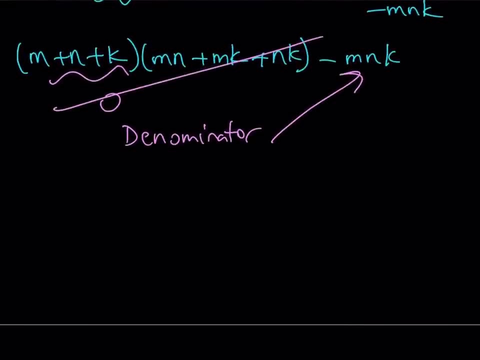 The sum of cubes, And then denominator is that one. So our expression is going to become then: m cubed plus n cubed plus k cubed divided by negative mnk. Of course we still need to simplify this. We're going to find a numerical value, But let's go ahead and look at our 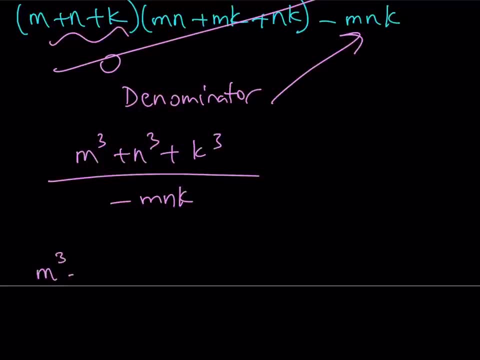 identity. I recently did a video on this one. I can also share the link down below. Remember we had this type of identity And we know that it's factorable. Especially, what we know is that this contains a factor Of m plus n plus k. we don't really care about the other factor, because what happens is m plus. 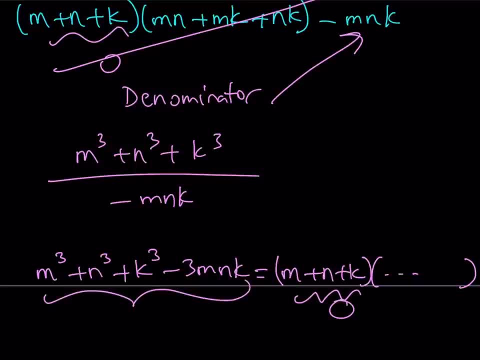 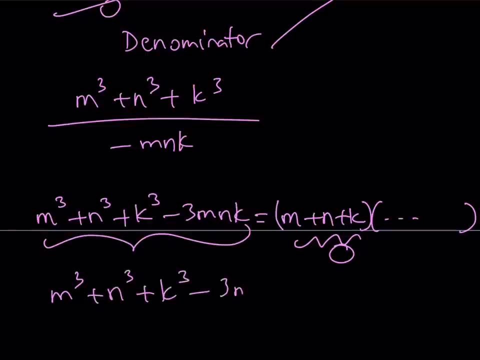 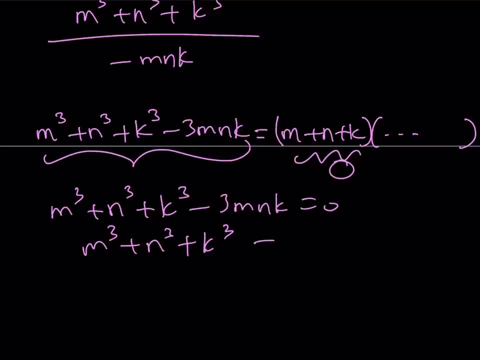 n plus k is zero. Therefore, this quantity will also be zero, which means that m plus m cubed plus n cubed plus k cubed minus three mnk is equal to zero, which means the sum of the cubes can be written as three mnk. Great. Now, in this expression, notice that we have the sum of the cubes in the 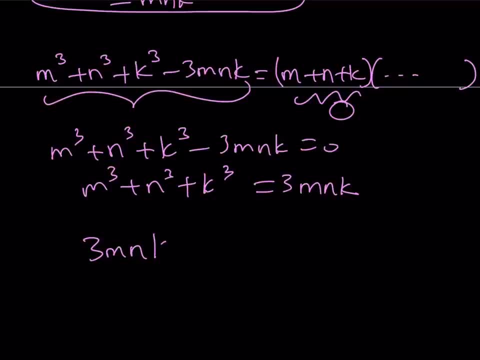 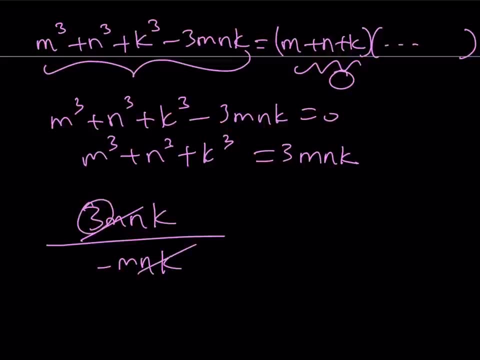 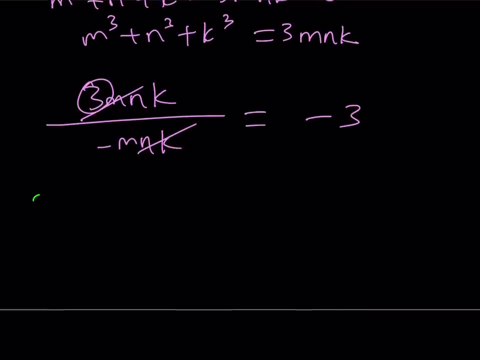 numerator. So we can replace it with three mnk And the bottom is negative mnk And they cancel out And, oops, the three doesn't And the answer is going to become negative three. So the answer is negative three. But let's go ahead and take a look at the second method, because the second method 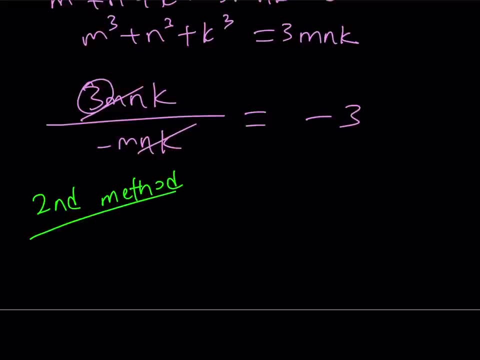 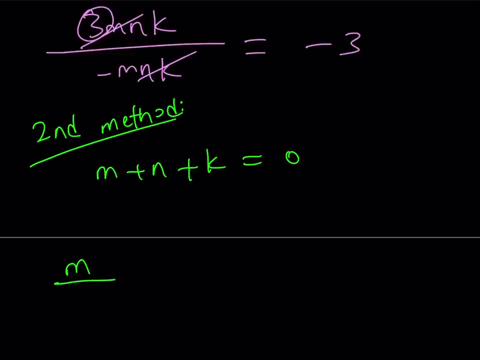 is more fun. The first method is a little painful. Why did I introduce that first? Because no pain, no gain. So let's go ahead and take a look at this Now. we know that m plus n plus m plus n plus k is equal to zero, And we're trying to evaluate something like this: m over n plus k. 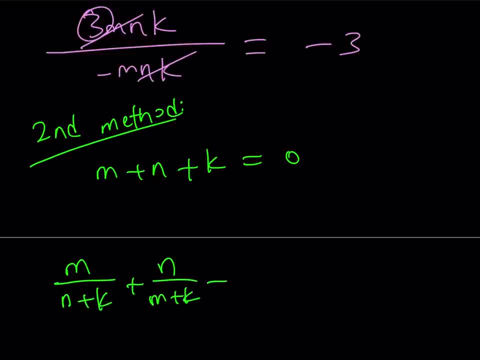 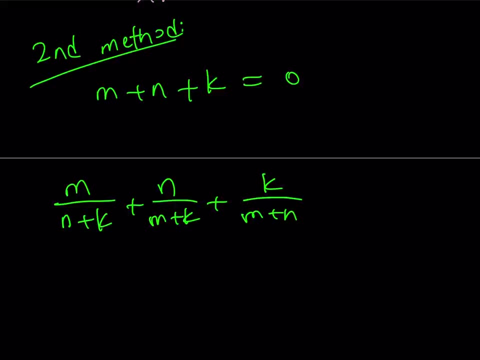 plus n over m plus k, plus k over m plus n. Now, what is that supposed to mean? Well, if m- the sum of these three terms- is zero, then you can basically say that n plus k is going to equal m plus k is going to equal negative m. This is going to be negative n And this is going to be 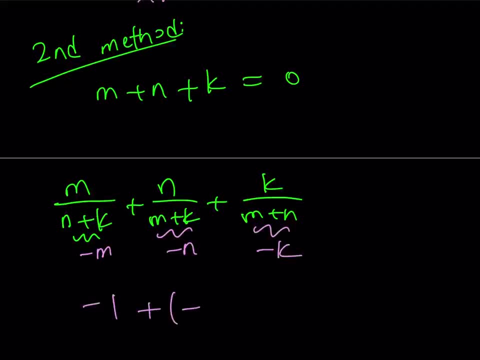 negative k, which gives us Negative one plus negative one plus negative one, which is equal to negative three. And this brings us to the end of this video. Well, thank you for watching. I hope you enjoyed it. Please let me know. Don't forget to comment, like and subscribe. I'll see you tomorrow with another video, Until. then be safe, take care and bye, bye.